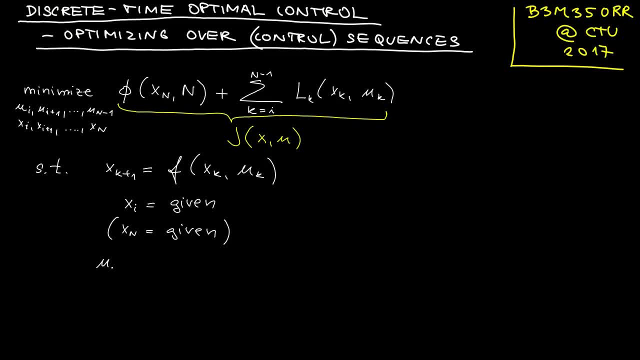 final state could be specified, in which case it does not make sense to include it in the cost function. Then, moreover, we can have some constraints on the, on the control signal and the state variable themselves. Formally, we can include these constraints on the initial and. 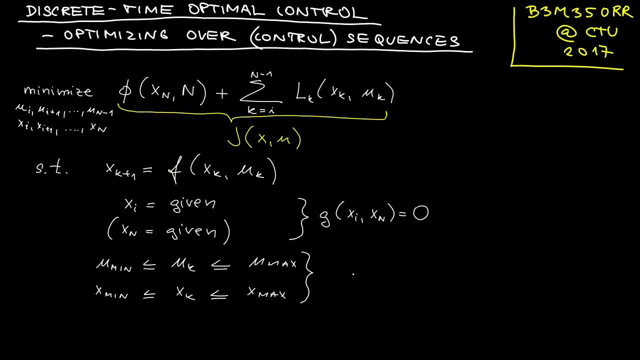 final state into some general equality type constraint g, and similarly the inequality type constraints we will label as h Now, since here let me remind you that the cost function is a function of both x and u, which are coupled through the state equation. therefore we call this approach 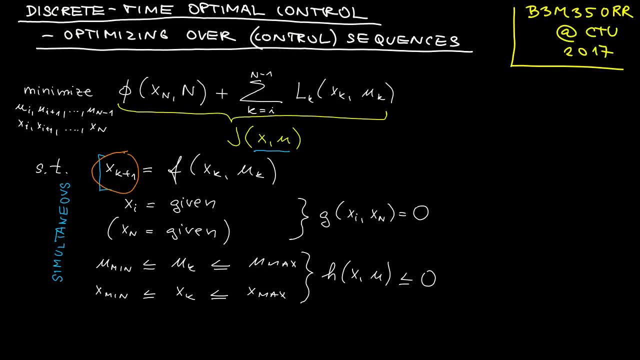 as a simultaneous framework. What we could, however, do is now we can use the state equation to actually eliminate the state variables From the cost function, and this will give us a new cost function- let's label it j- tilde- which will only be function of u and possibly x- zero, or in fact it should be x- i to keep the notation. 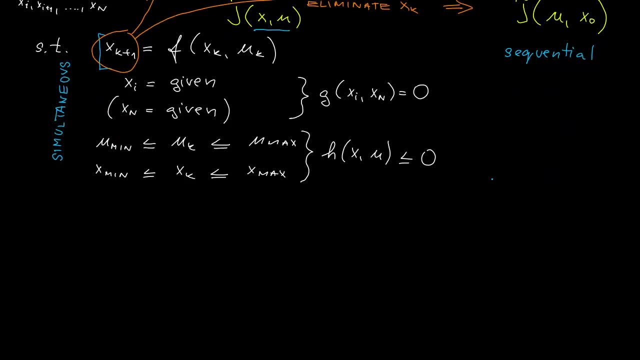 And this framework is. this approach is called sequential approach and I will illustrate it in a while by means of of an example In particular. we will consider linear system, we will consider quadratic cost and we will consider linear system. Then, for the following SLOJ parameter, we willimatil mobility, SLO and we will consider the so-called 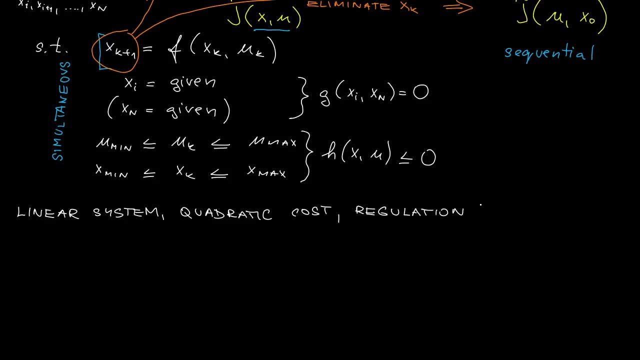 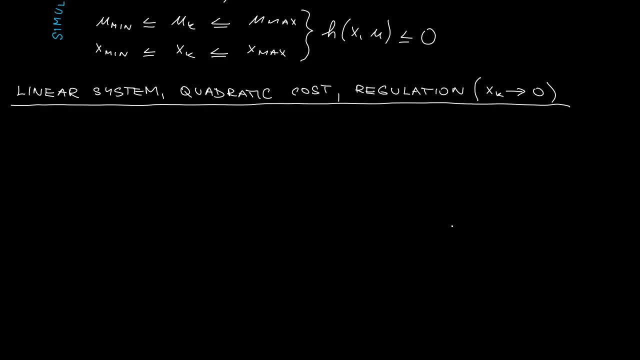 regulation task in which the goal is to bring the state to zero. Now the cost function will look like this: it will be one half of the term corresponding to two. сыl enfío como propósito final e a hakko fikí de sum of the terms corresponding to two. and controls throughout the interval of controls. vinatio aśable y que aśable y que se repite. another interval, As I, for example, divide the whole number into two peaclooking values to show you now theuring that the next stepлон 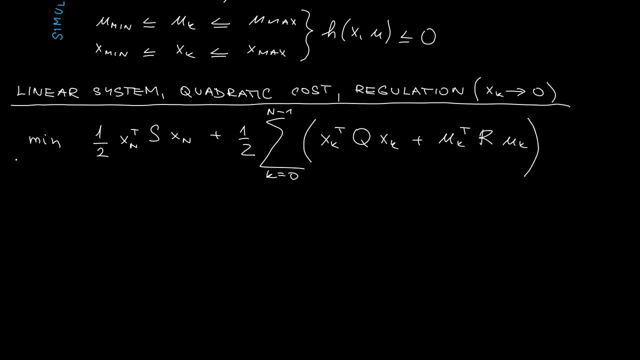 is none the numerator and negative Shock traveling example form. the content violation of is a n. caucus erkennen, an control. and now the interval of control starts at zero and goes to, goes to n, but note that u is only considered at n minus one interval, because that's the only time when it influences the state. 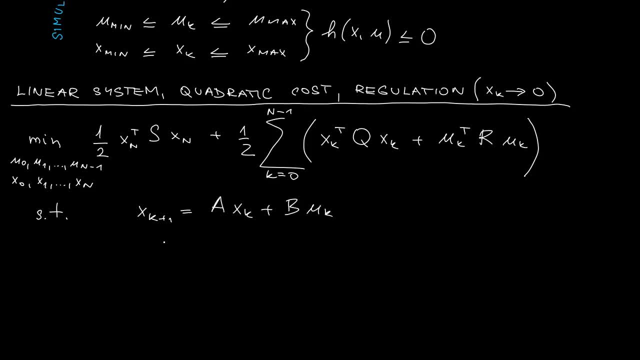 at n. now the constraints come in the form of a classical state equation, and the initial state is given first. we will not consider constraints here. now let's what we will do in the following is that we will take all these state vectors and stack them into one long, super long column. 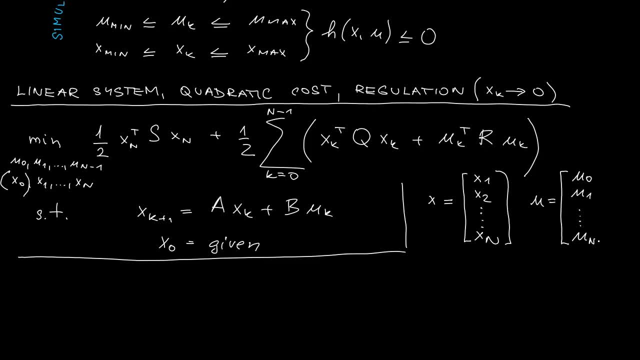 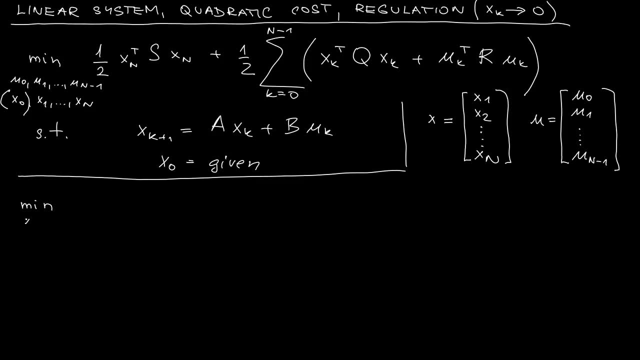 similarly with the control signal. so then we can write down the cost function in the following way, explicit way. so the cost function, so the term corresponding to the state, at the final time will have this long X vector transposed. in fact, I in I forgot to include the transposition signs with each. 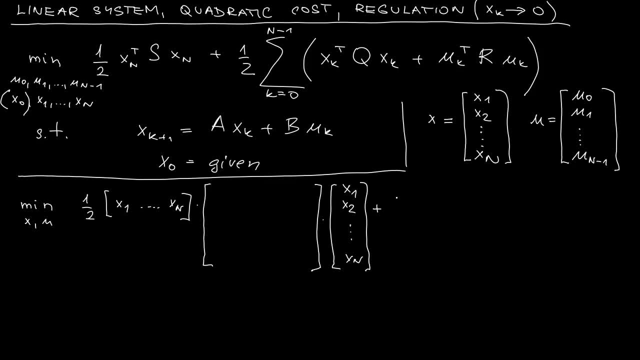 individual X's and then here the, the waiting matrix will look diagonal, with the last element corresponding to the penalty for the final state and similarly for for the controls. here also the weighting matrix will be diagonal or block diagonal, containing our matrices on the diagonal. and finally, i will explicitly here separately state the term. 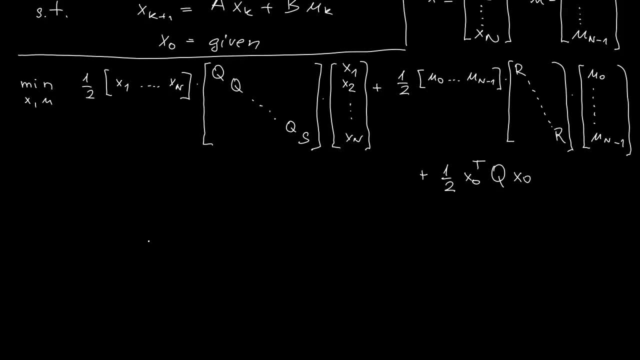 corresponding to the initial state. its role is certainly different from the roles of other, from the roles of states at other time instances, in that it's fixed. now the constraints here, it may take just a few moments for you to recognize that this is indeed how the state. 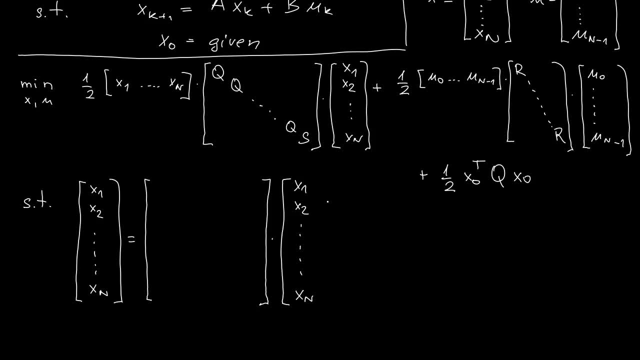 equation could be written down. so here i will have some matrix: not yet specified: times the long stacked vector x, plus another matrix times long stack, the vector of controls, plus yet another matrix times the state at the final, at the initial time. so now, how about the matrix that relates the states? it's in fact it looks like this then: 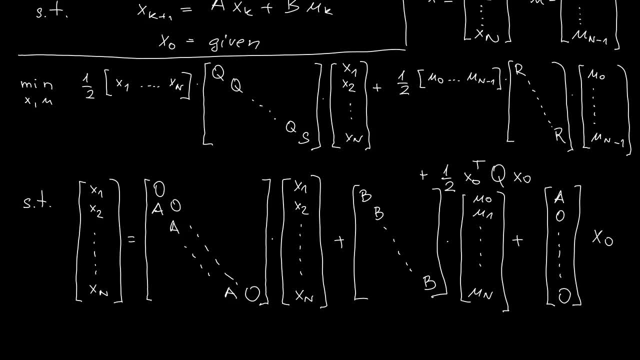 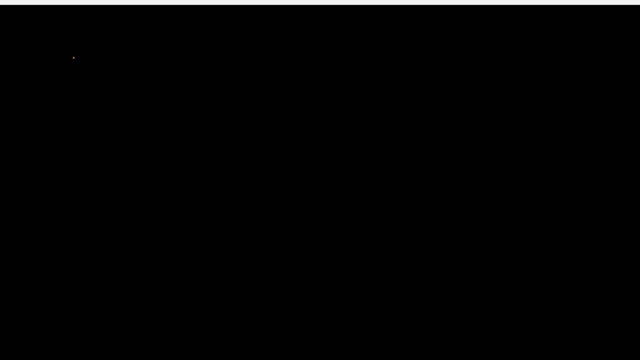 yeah, so check it out by yourself, and i will label these matrices and as q bar, r bar, this will be a bar and this will be b bar and possibly this a naught. now this, in fact, could be regarded as a quadratic problem already, but if you, if you like, we can now combine. 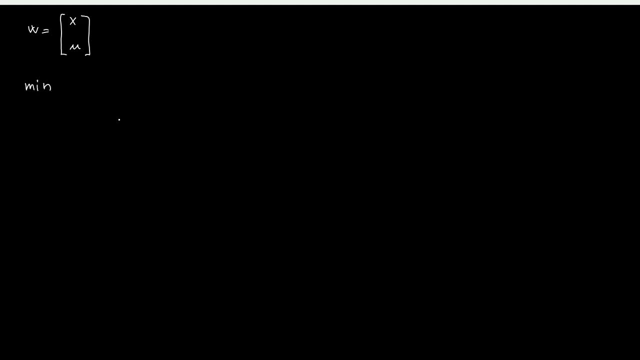 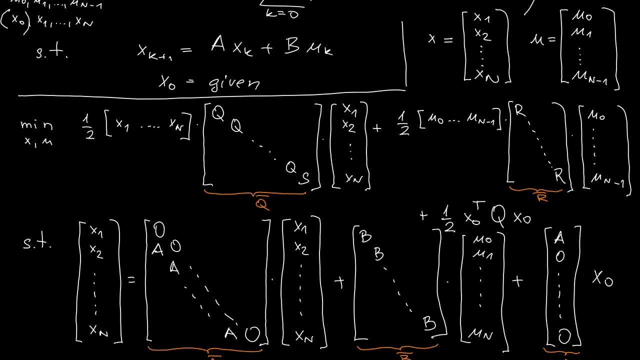 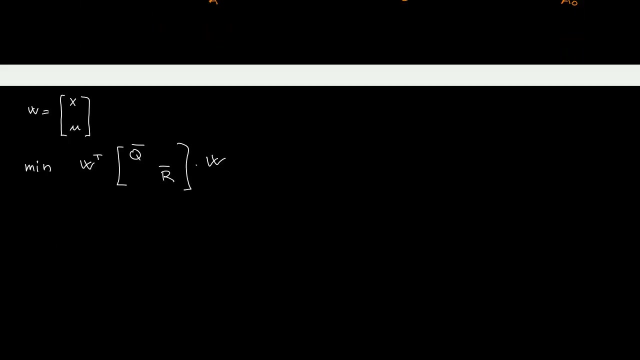 the states and the controls into just one long vector, and then we will formulate the optimization as really minimization of this pure quadratic form. how about the constraints here? yeah, i will. i will in fact disregard the term corresponding to the matrix that relates to the initial state here, because it's just a constant offset. and how about the constraints here? 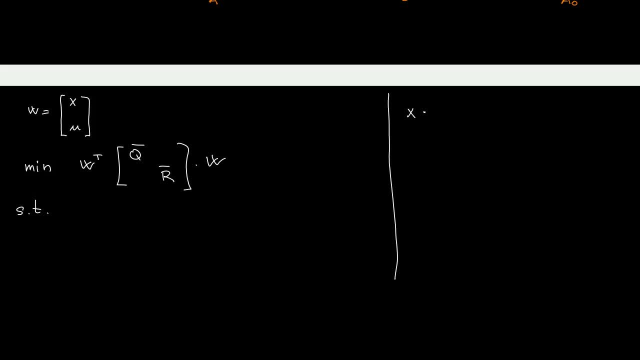 in order to see how they look like. let's now write down explicitly here that the long vector x can be expressed like this: this is what we had up there now, moving everything on the left hand side- this is what i get- and finally stacking together x and u in one. 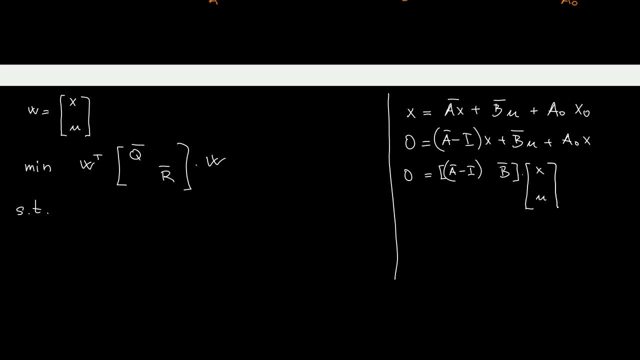 combined vector w. this is what i get so clearly. clearly, this is a linear constraint, or constraint in the form of a set of linear equations. perhaps we can label this as a double tilde times w is equal or plus b tilde is equal to zero. so clearly. 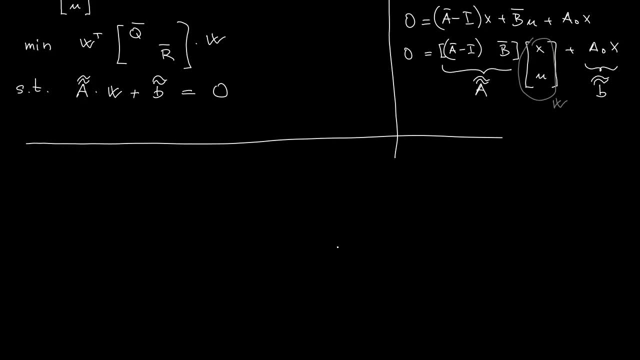 linear constraints, and this renders our problem perfectly suitable for solving by quad proc function. now i've mentioned up there that we can also eliminate the state variables altogether. so let's, let's do it now. either we can write now the the long x vector as a function of the long u vector and the initial state, or, if you want, and i can do it in this: 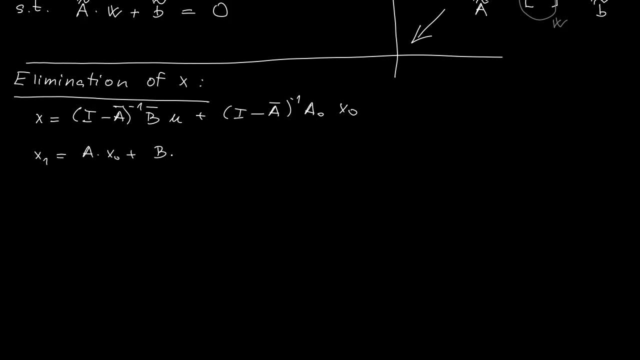 vector form or we can do it in a step-by-step way. So first I write x1, then x2, and obviously x2 depends on x1, which I can express from the equation above. I think this procedure is pretty much familiar to you. Obviously, what I 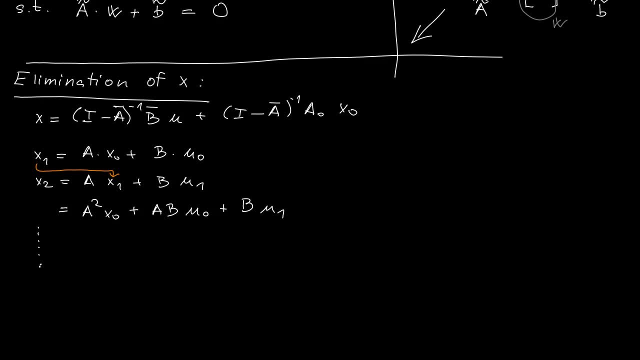 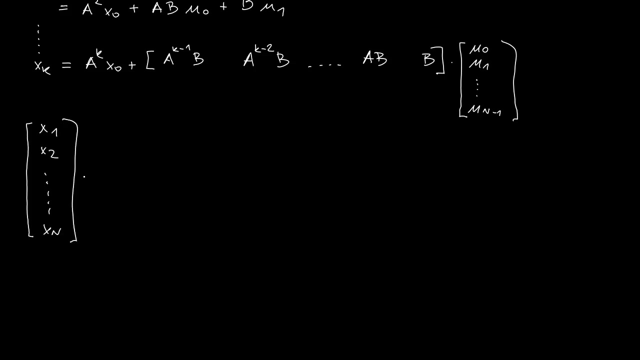 will do now is: I will express x at some general time. k and this is already pretty obvious where we are heading. So if I now proceed by stacking all these state vectors into that one long vector, this is how the relationship between this long x and long u looks. 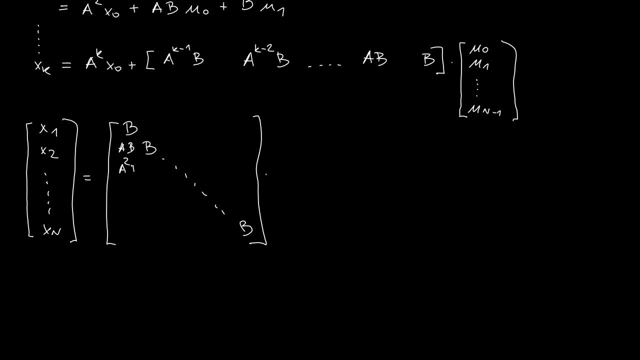 You can again check by yourself. Now you can perhaps recognize here really pretty much familiar pattern. Doesn't it look like I mean this block lower triangular matrix? doesn't it look? looks like a controllability matrix. Let's label this as a C bar and the other. matrix as C bar. Let's label this as C bar and the other matrix as C bar. Let's label this as C bar and the other matrix as C bar. Let's label this as C bar and the other matrix as C bar. Let's say a hat. and now from this I can substitute into, into our cost function. 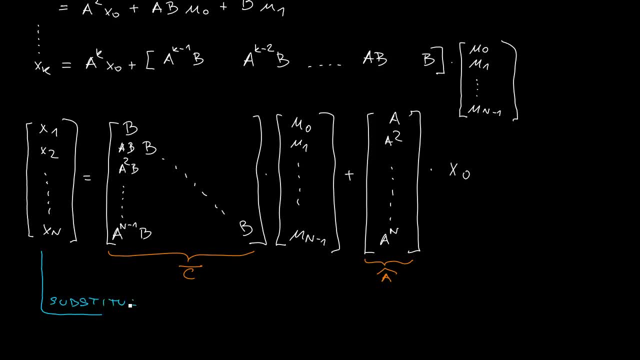 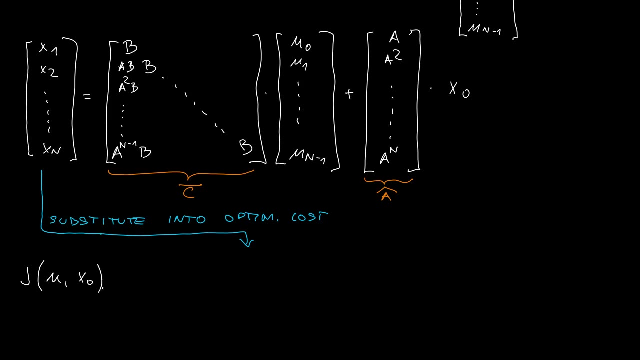 say a hat. and now from this I can substitute into into our cost function, as we derived above in this format, using these long vectors. This will obviously be new cost function. So here I'll substitute for the state from which I can inherit the job product from the cost function. 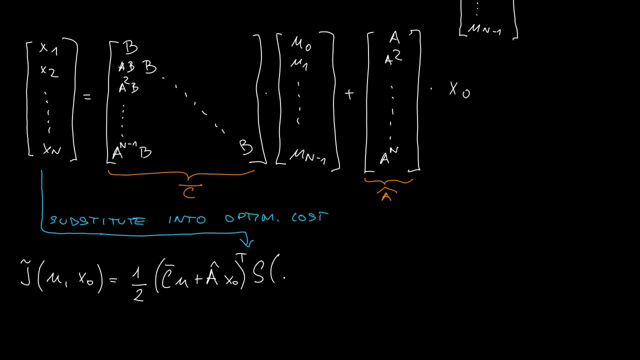 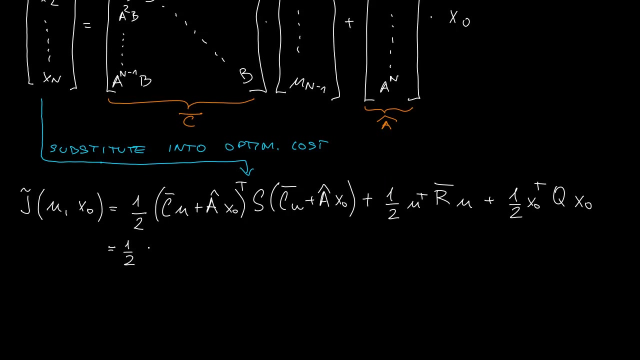 vector at the final time. this actually sorry. no, not at the final time, but the whole, the whole vector. similarly, the term corresponding to controls and, finally, the term corresponding to the initial time. now, let's, this now becomes somewhat technical, but let's go through it in order to get some, some final 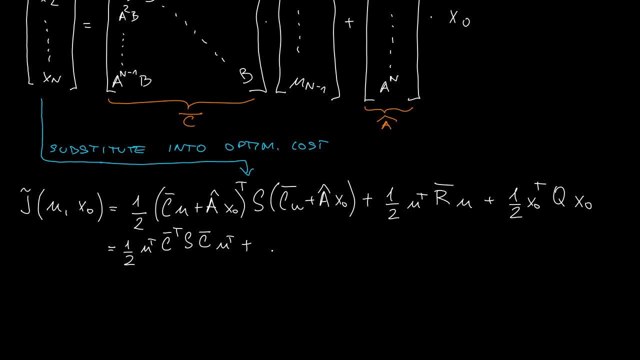 results. so I will multiply out of the brackets and combine all the terms that could be combined. so let's give it a few more, few more moments, all right? so now what I can do is now I can combine the terms that that are related, so all the terms that are related to the initial time that are 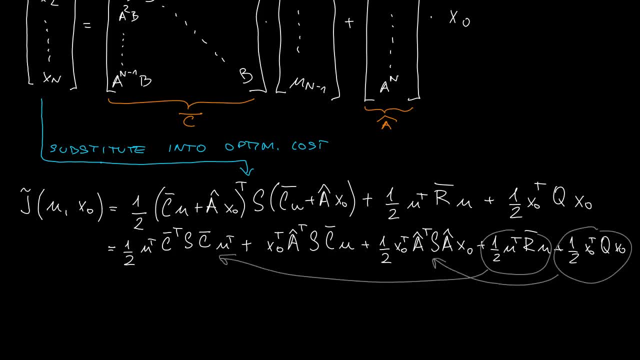 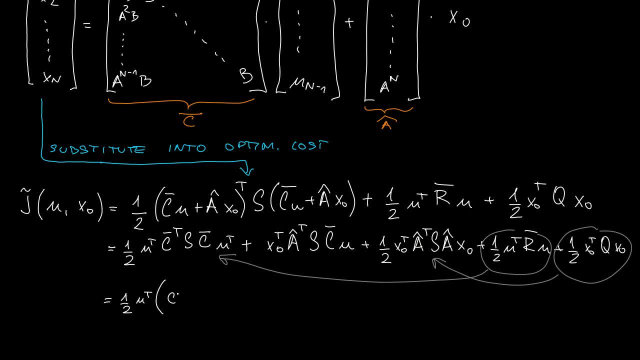 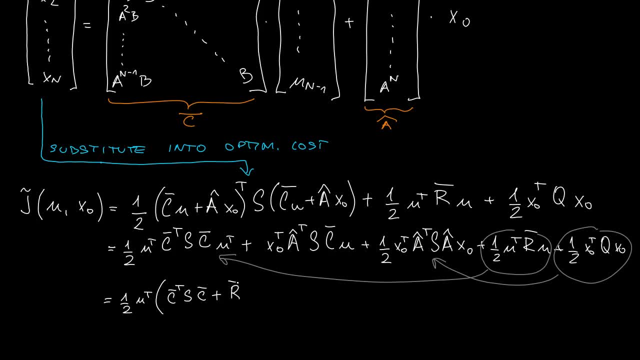 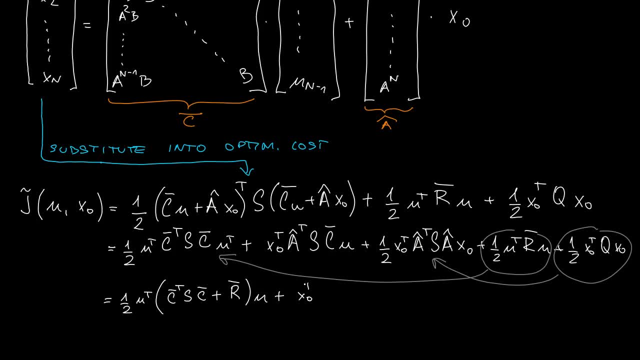 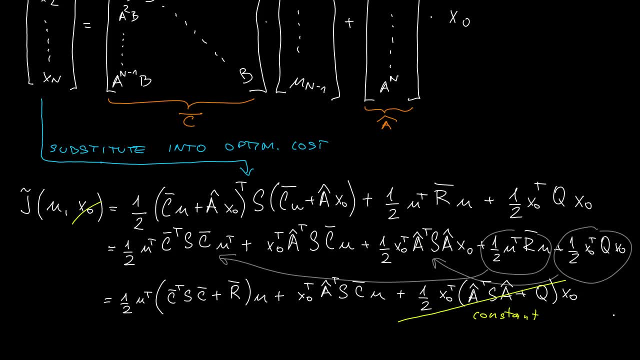 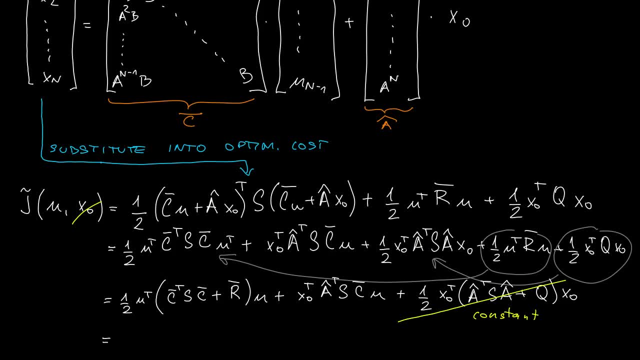 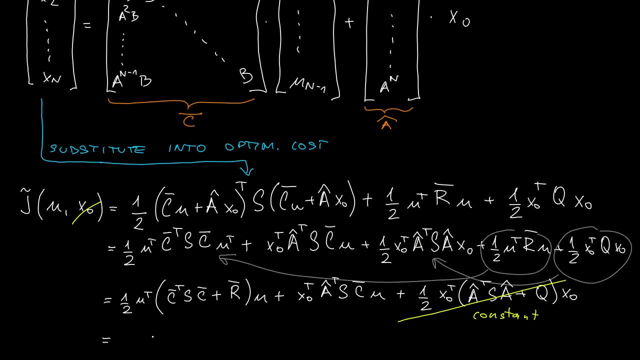 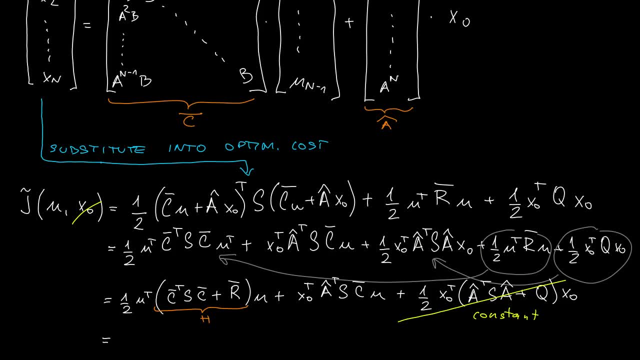 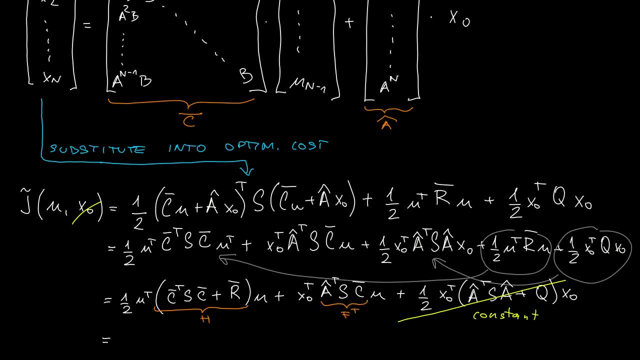 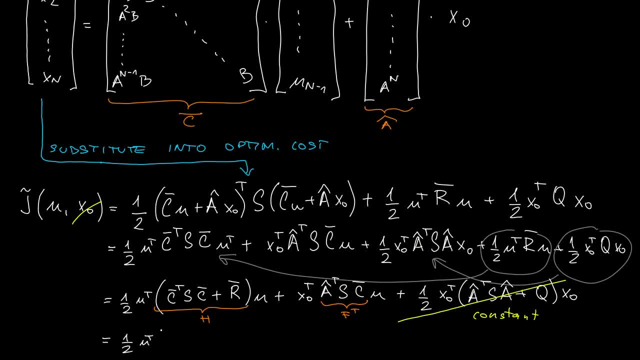 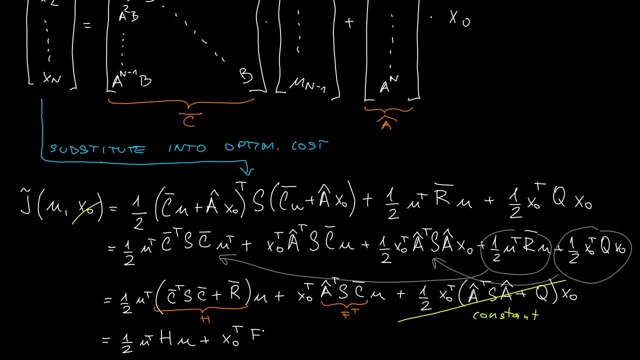 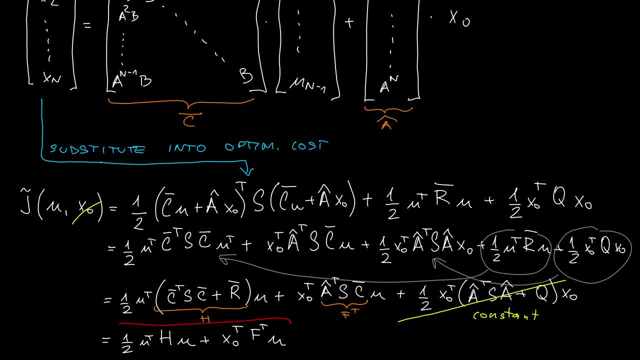 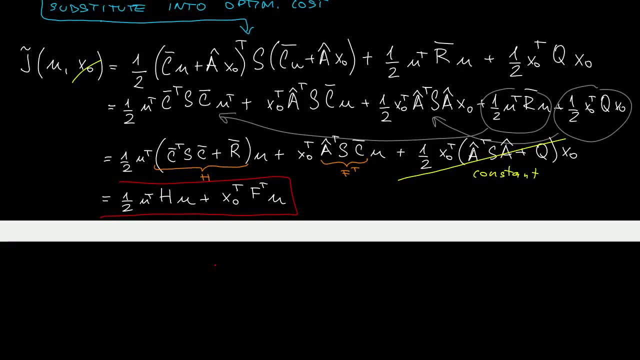 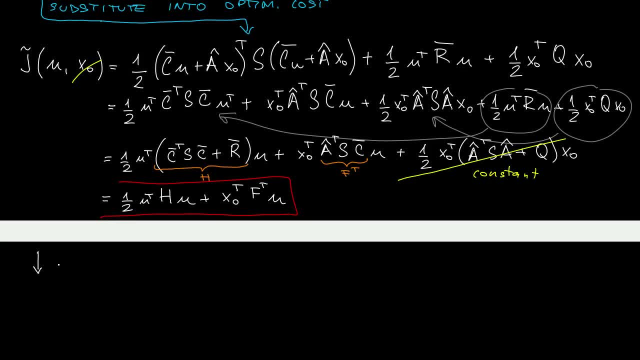 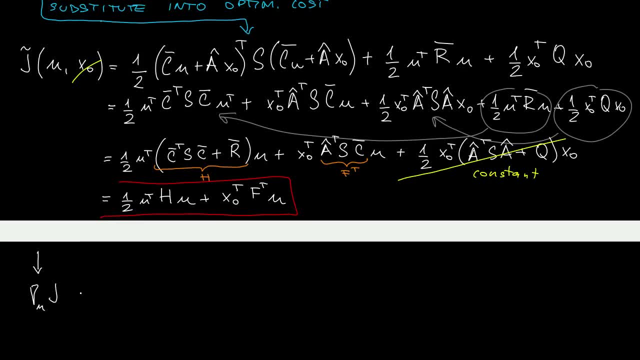 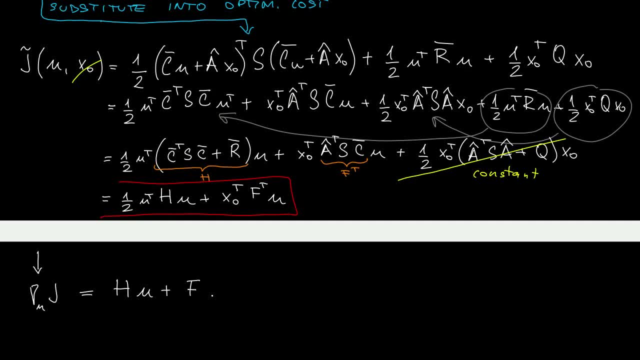 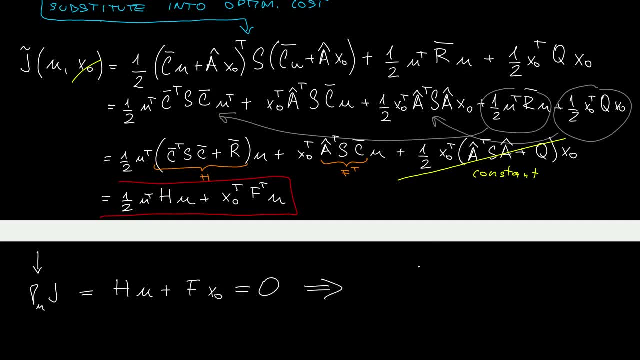 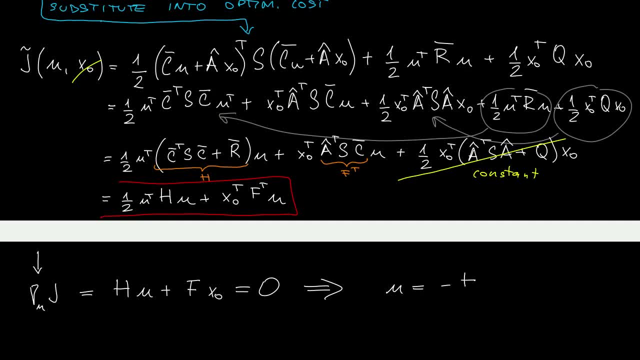 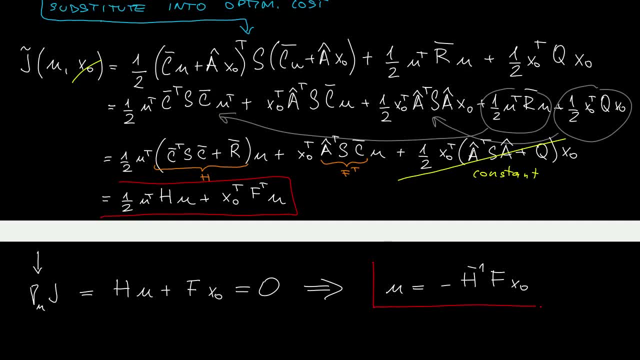 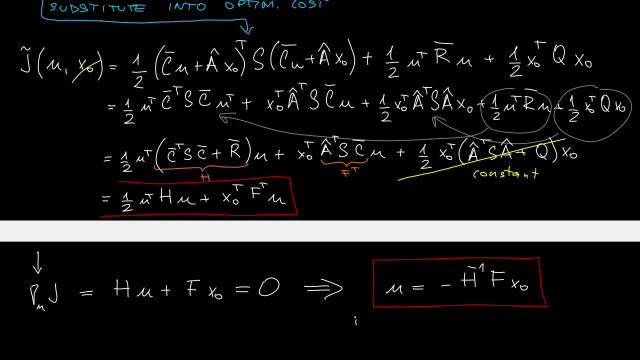 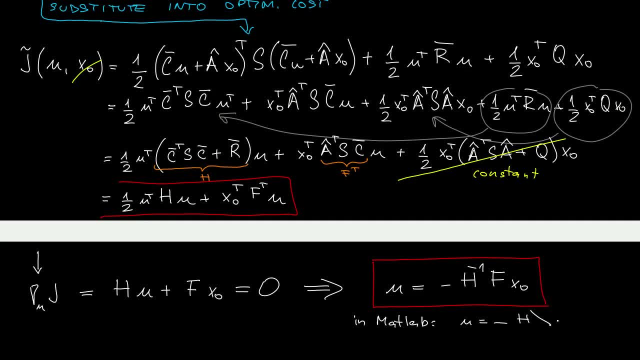 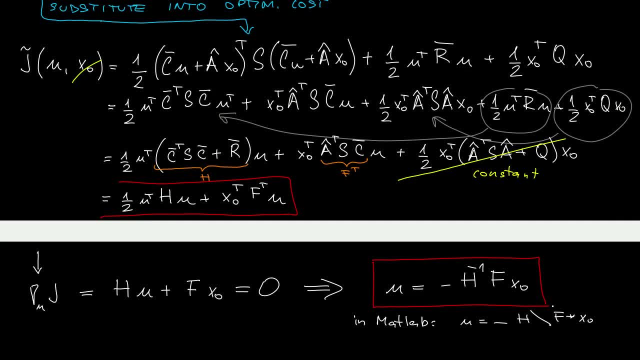 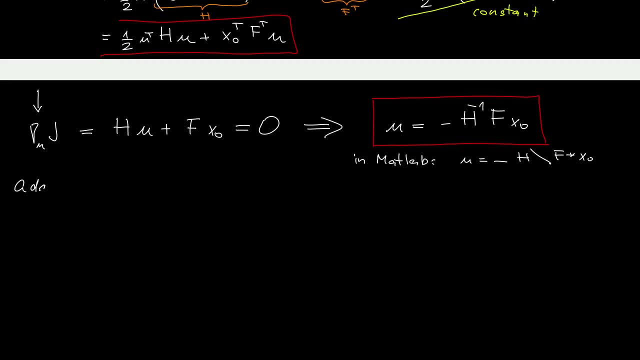 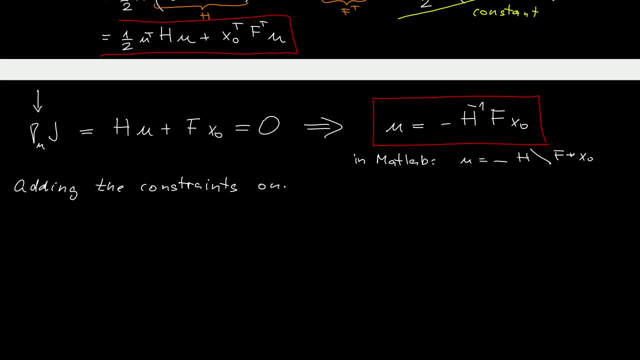 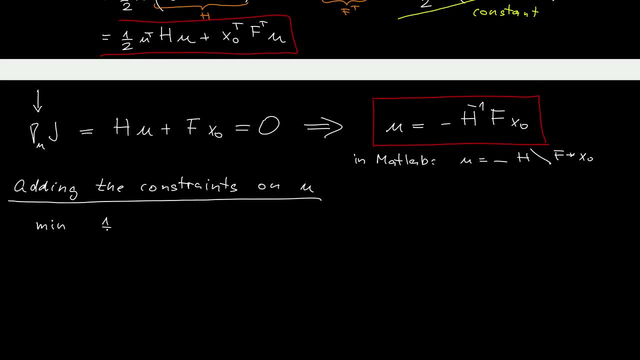 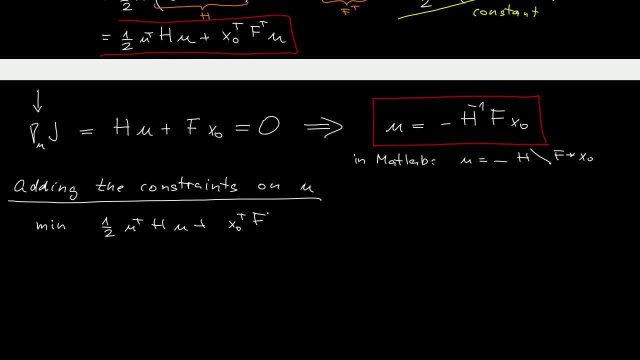 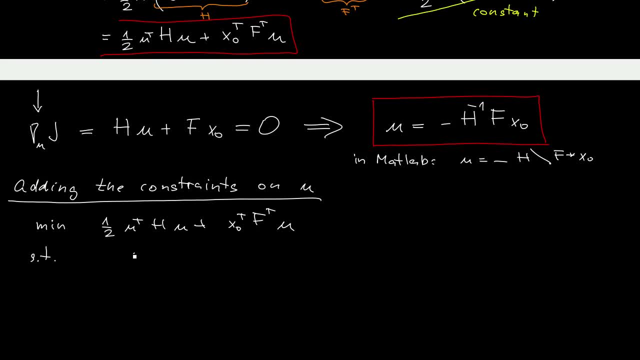 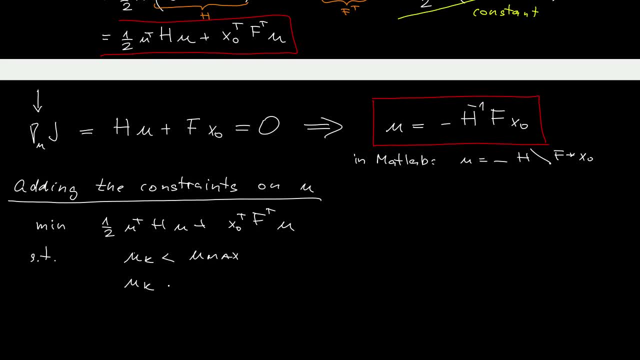 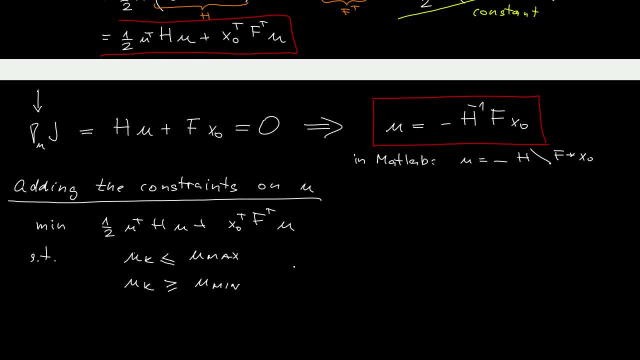 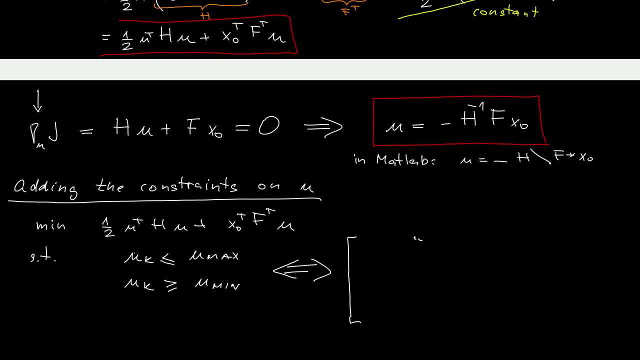 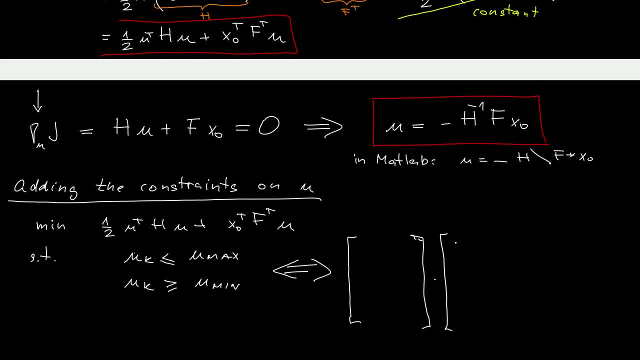 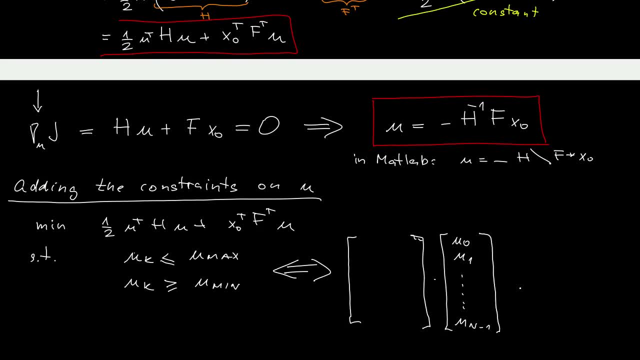 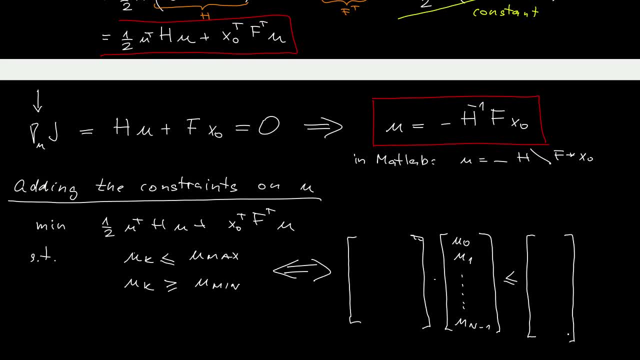 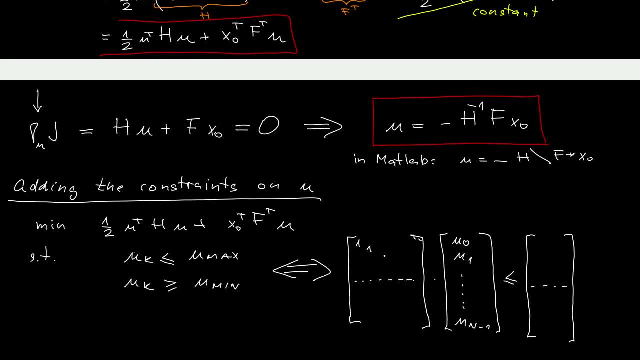 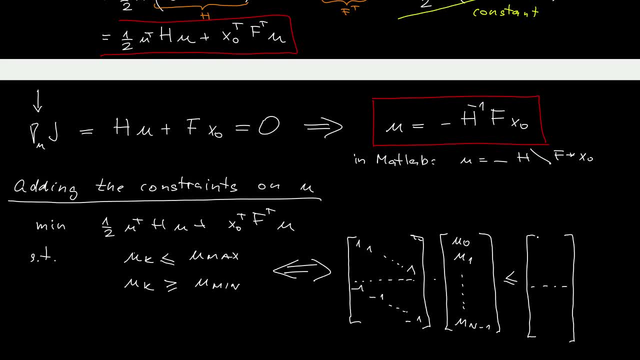 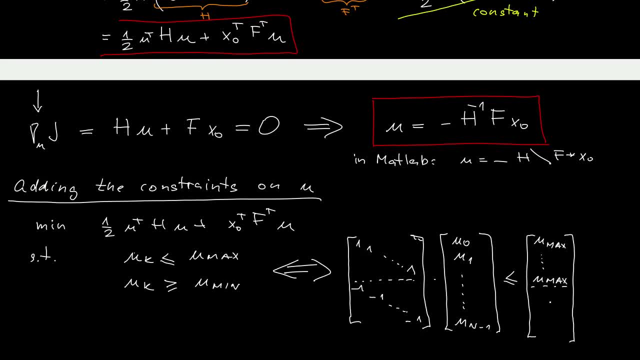 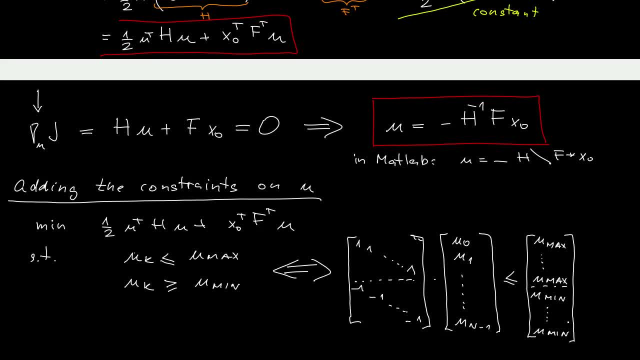 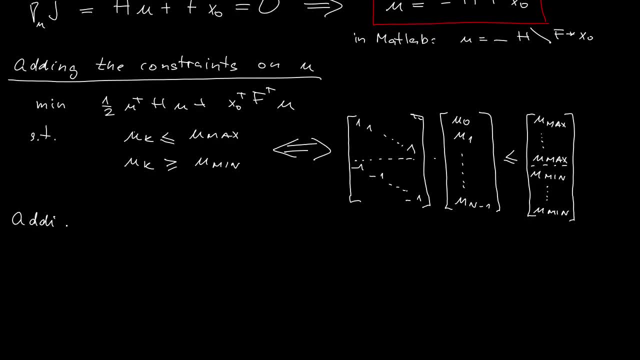 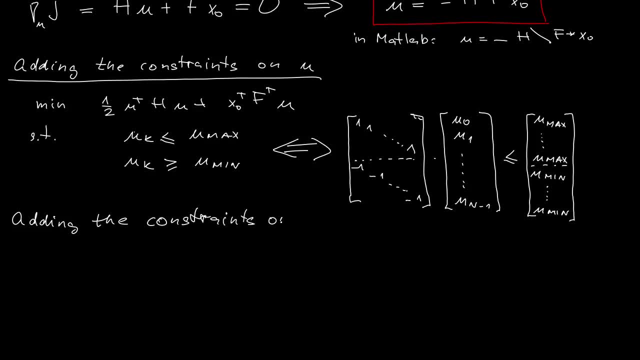 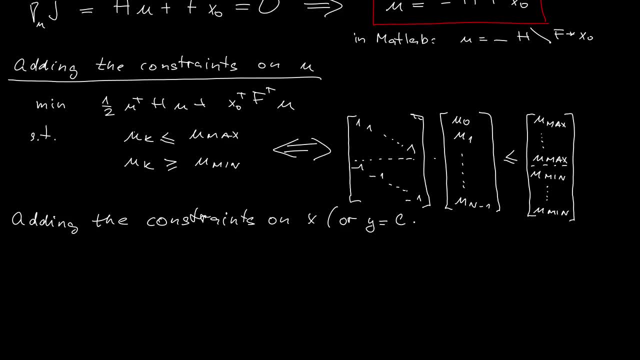 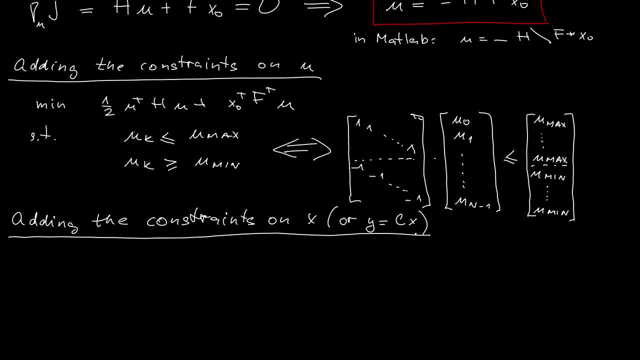 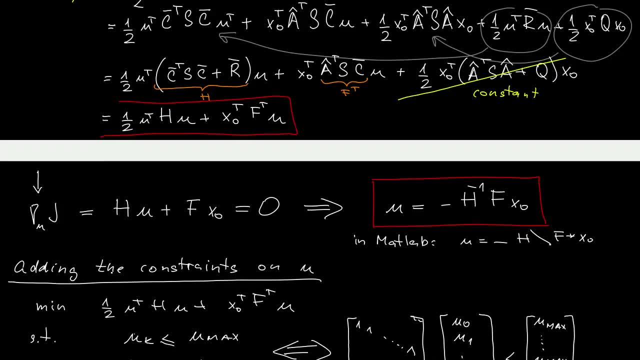 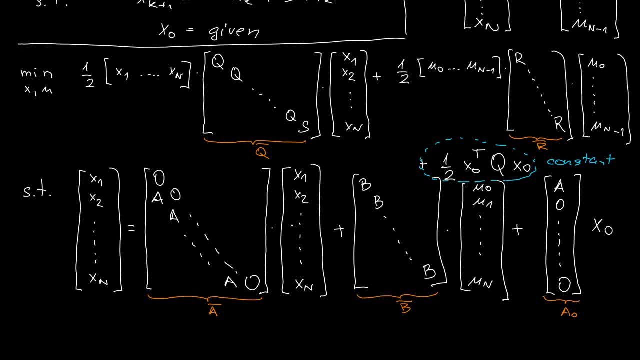 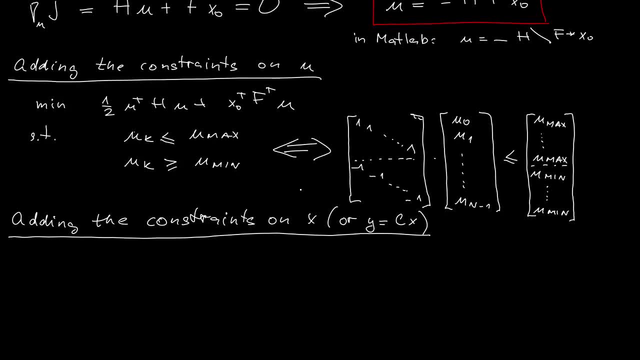 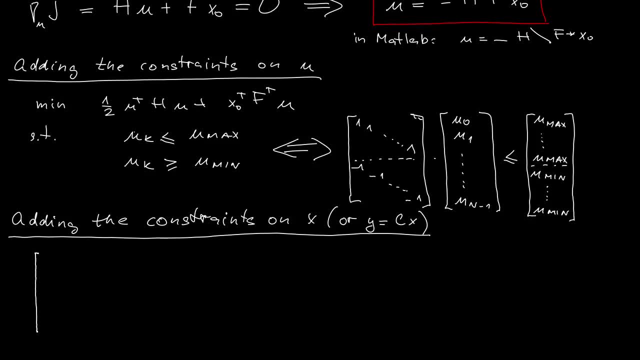 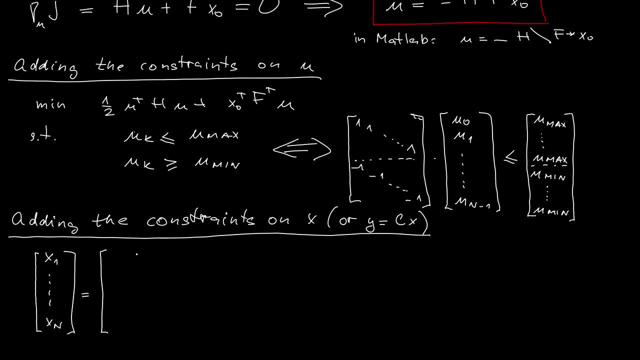 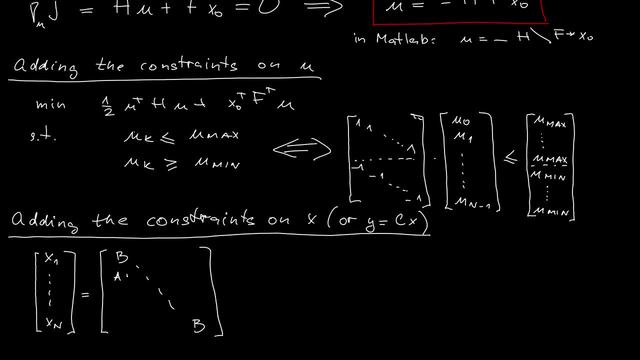 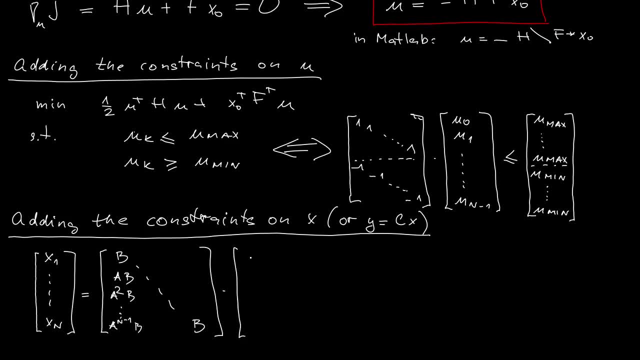 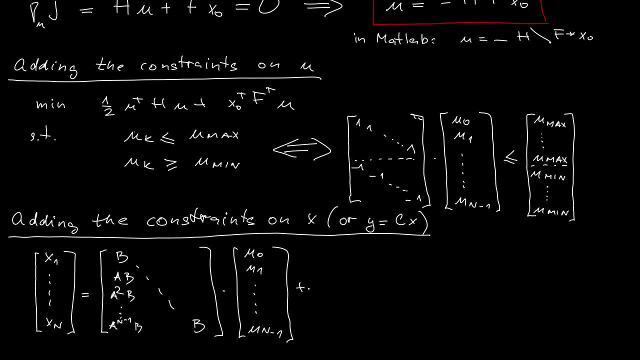 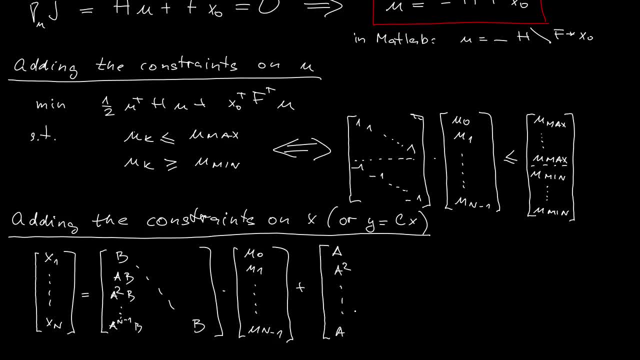 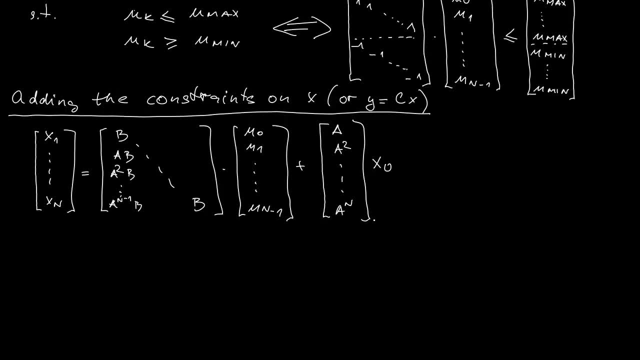 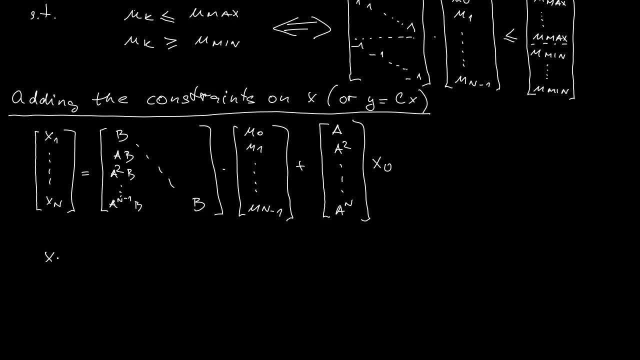 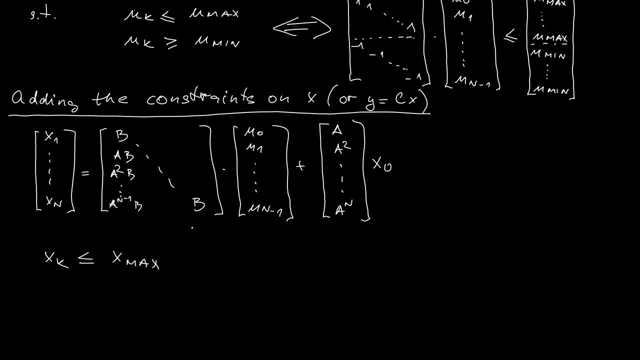 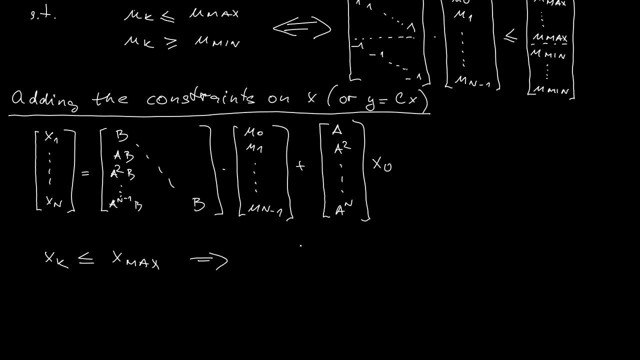 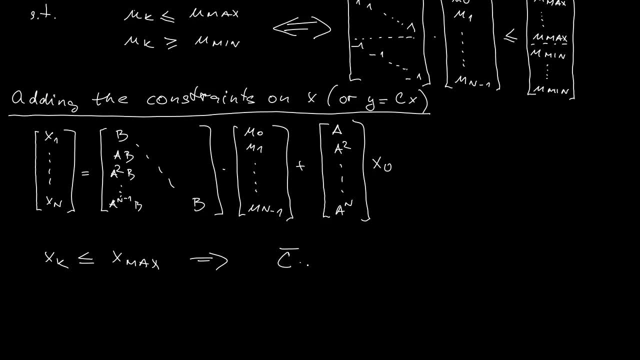 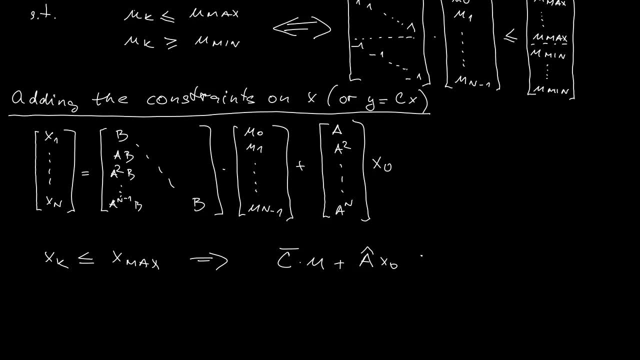 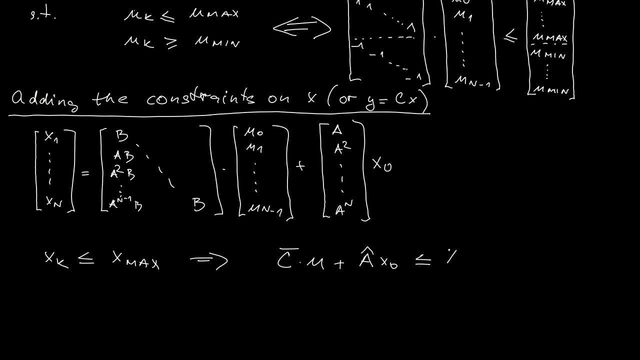 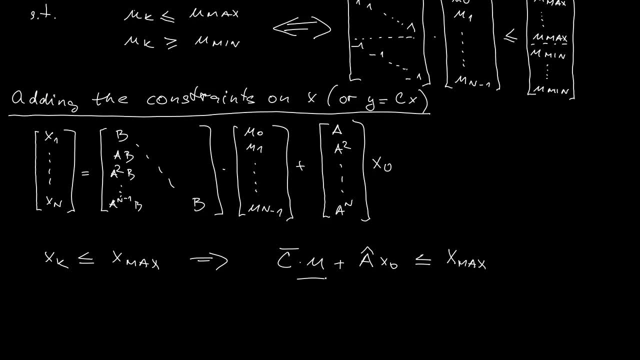 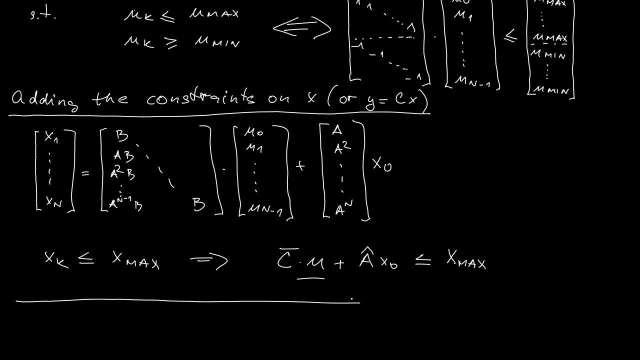 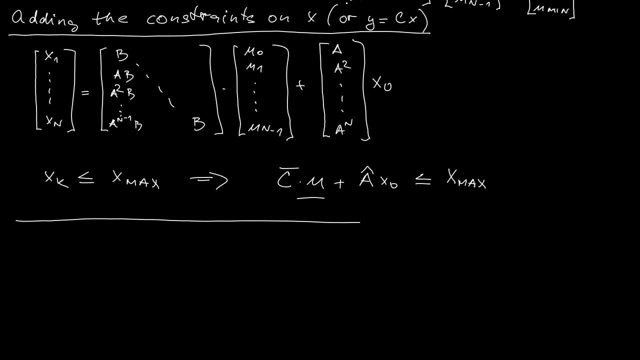 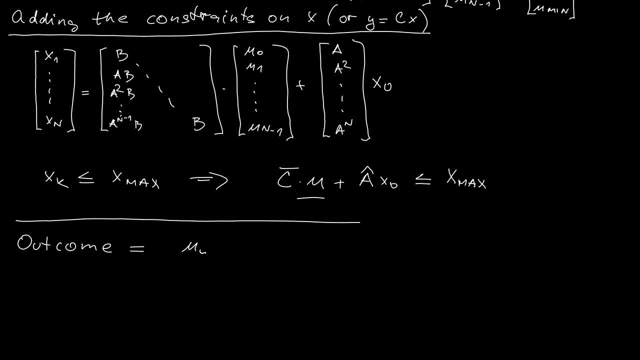 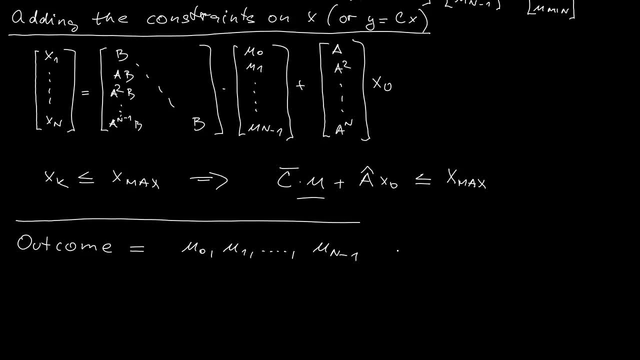 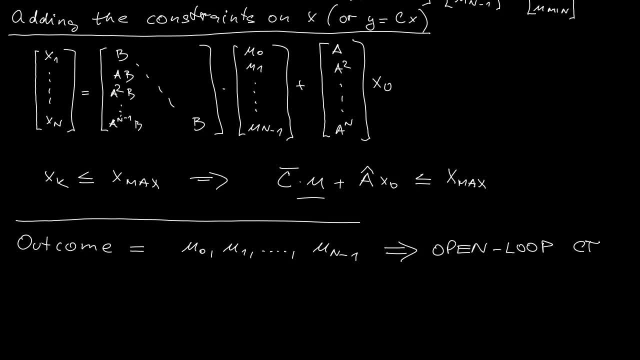 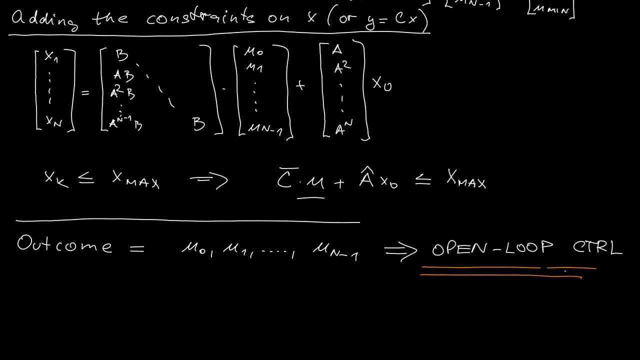 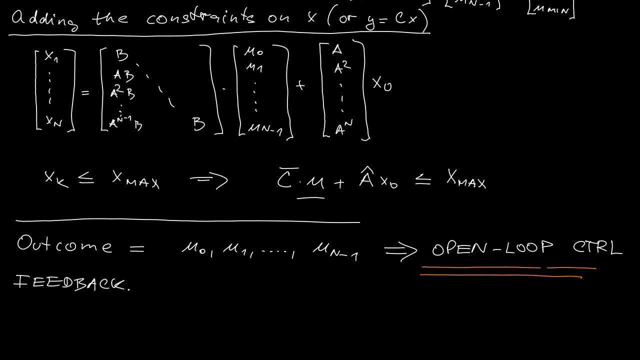 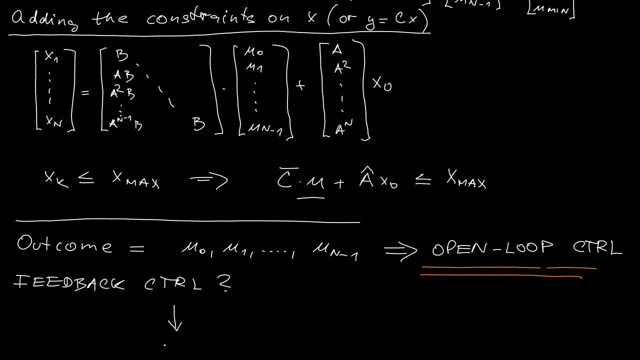 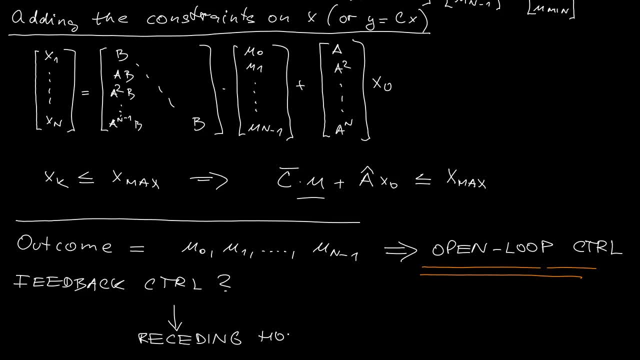 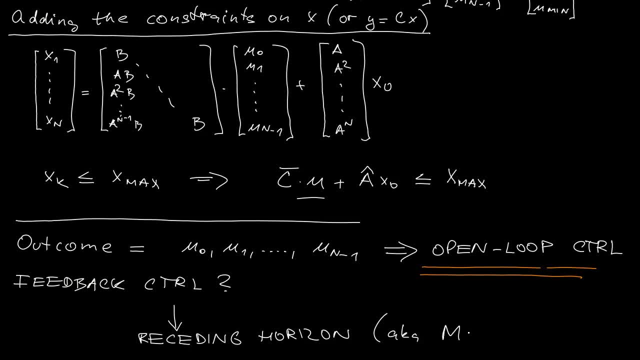 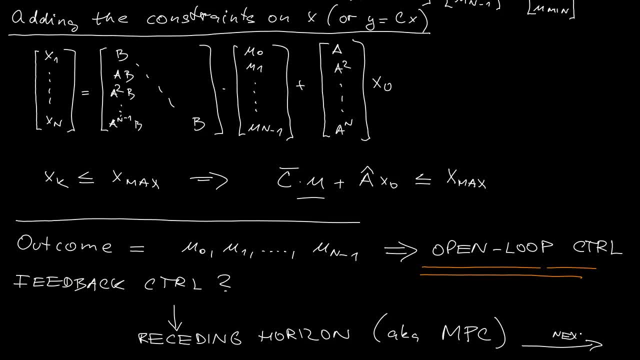 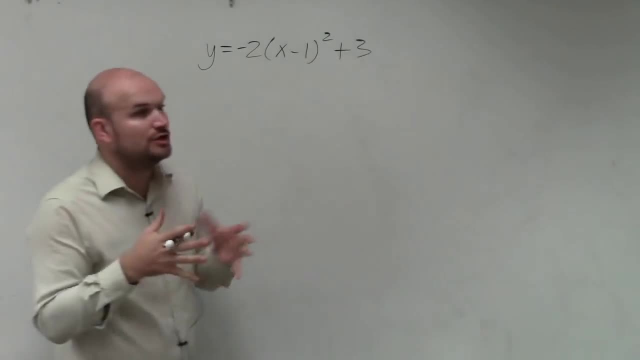 So in this example, basically, ladies and gentlemen, they're asking you to go ahead and graph the function right? So what we discussed in this class, or what I told you guys to write down for your notes, was what the parent graph looks like. y equals x squared. 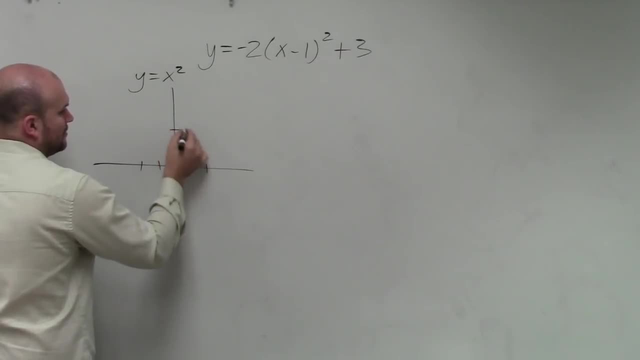 And I gave you guys the points and the table for what that graph looks like And you guys can see that it's different than the v-shaped graph for absolute value that we talked about. This is called a parabola and it's the u-shaped graph, correct? Now the important. 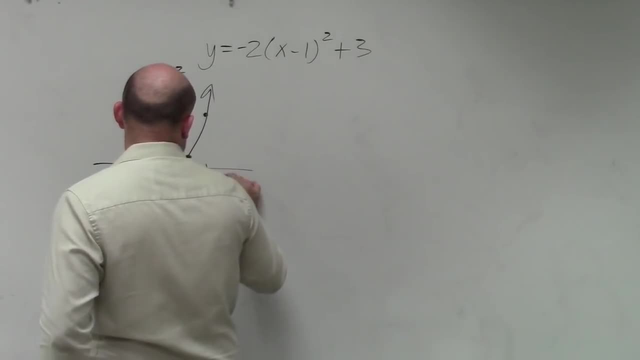 thing about this is remember: the vertex was at 0, 0.. And the axis of symmetry, the line that the graph is symmetrical about, was at x equals 0.. Then what we did is we learned a new form of. 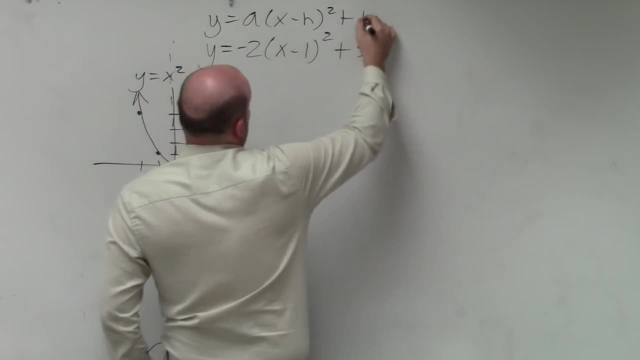 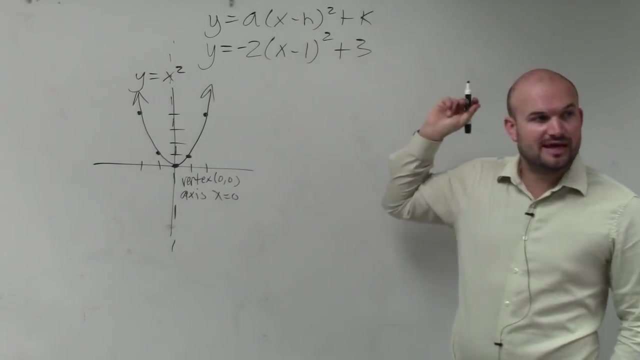 an equation which is called the vertex form, And vertex form had the a, h and the k And you guys can see that we have values for each one of those letters. x and y represent any point that's on the graph. So what I said that was nice about vertex form is: you can